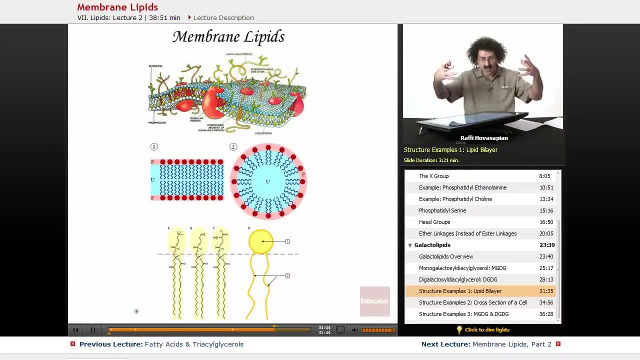 Okay, so first of all let's take a look at a nice general. we're going to work our way down. we're going to look a little bit deeper in magnification. So we have our general lipid bilayer. this is a nice cell membrane. we see some integral proteins. we see the lipid bilayer. we see our. this is our top layer here. 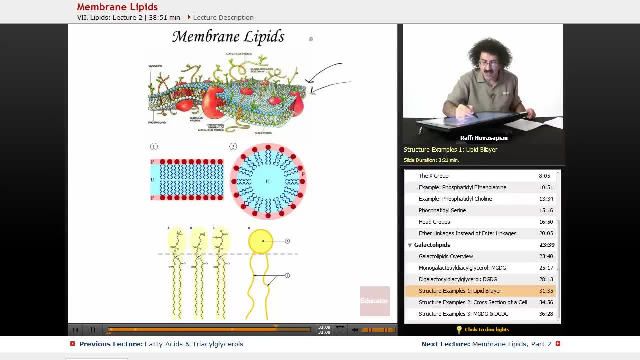 this is our bottom layer there. so we have outside of the cell, we have inside of the cell, so we would call this the outer leaflet, we would call this the inner leaflet, and you can see these little blue things. this is our head group and you can see the tails a little bit. so when we magnify this now we're going to come over to this level. 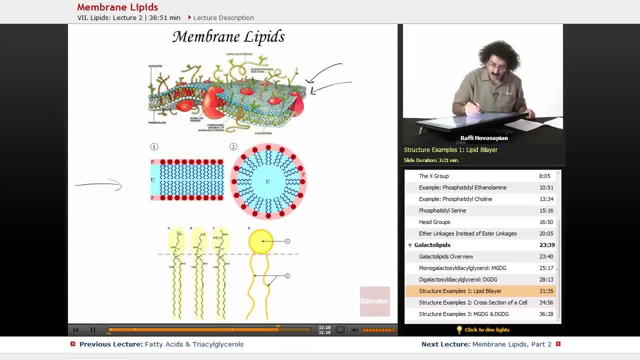 So nice cross-sectional view. we have our head groups. these are the head groups. these are the tails. notice that we have the head groups. these are the tails. notice that we have the tails. there are two tails attached. so these are our glycerophospholipids in general. you have the two fatty acid tails attached. 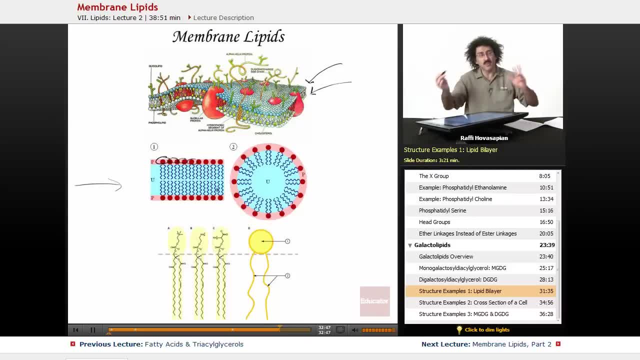 they're going to arrange themselves like this again, because polar with polar, non-polar with non polar, these are non-polar tails attaching to non-polar tails, the outer leaflet, the inner leaflet. this is something called a mesel. oftentimes they will arrange themselves. one layer of these can arrange itself in a circle. 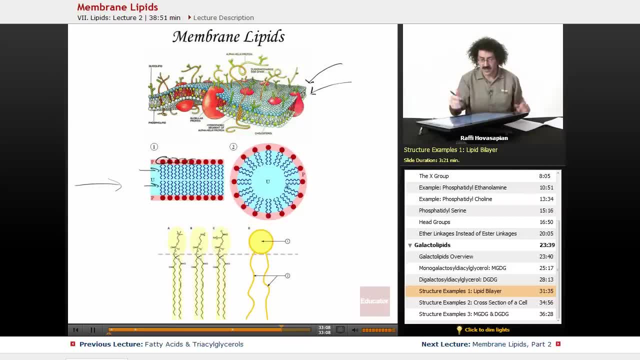 and create a famous, beautiful a name for itself. this little container, if you will, where the inside is actually nonpolar, the outside is polar. the soaps and detergents that you use they often do it like this: they trap the oil inside here, but they interact with water outside. 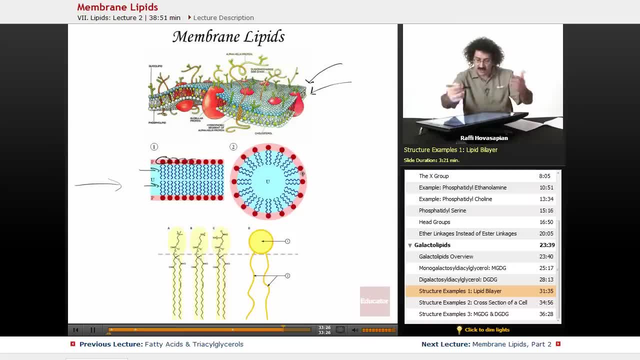 here, because these things are polar, okay, so now let's magnify a little bit more. now we have an idea of what it is that they look like. so this is the what you might call the well I separation. this is, this is what they're showing. so what you 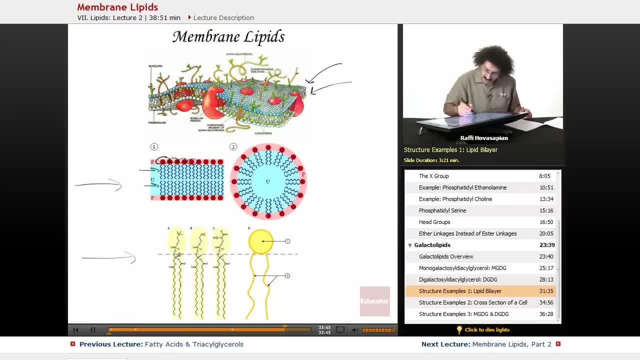 have here in this particular case. so we have our glycerol right there. okay, this is our glycerol. we have one of the fatty acids attached. we have another fatty acid attached- here's our phosphate group- and then of course our glycerol. and then of course our glycerol, and then of course, our. 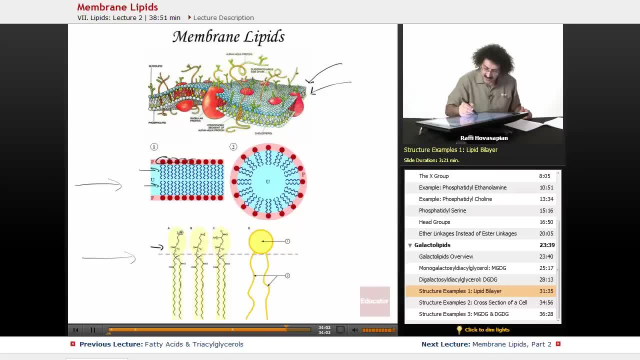 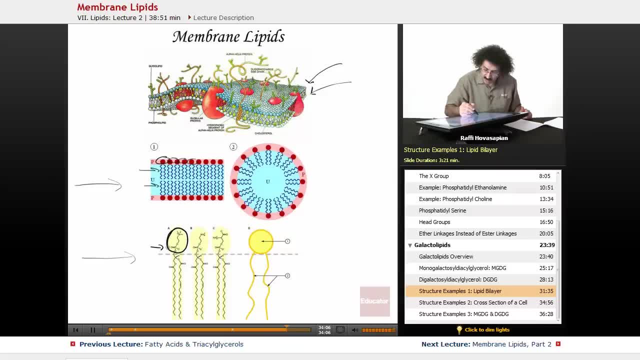 have CCN, we have CCC, so this is have CCN, we have CCC. so this is choline. so this is our polar head group, choline. so this is our polar head group, choline. so this is our polar head group. okay, that is that and these down here. 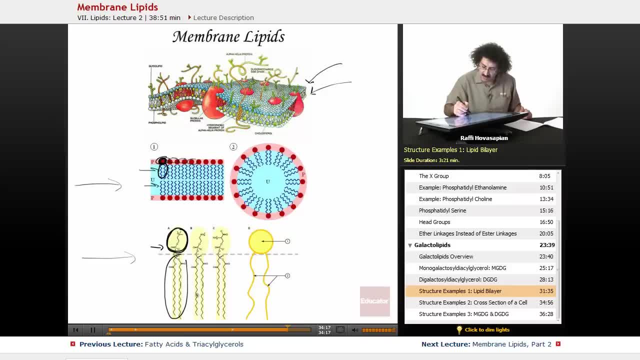 okay, that is that, and these down here. okay, that is that, and these down here, that's that in this particular case. same, that's that in this particular case. same, that's that in this particular case. same thing, except we have ethanol amine. thing, except we have ethanol amine. 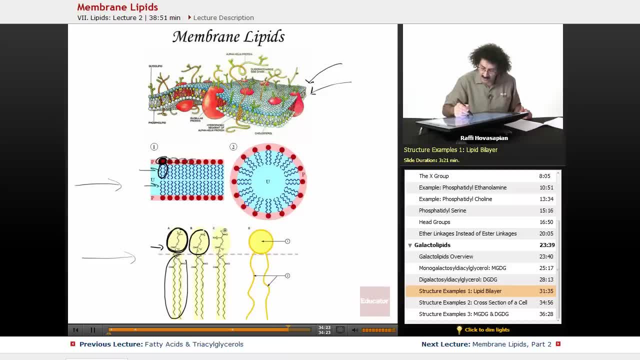 thing, except we have ethanol amine instead of choline, but we have our instead of choline, but we have our instead of choline. but we have our phosphate, and here we have our serine, so phosphate, and here we have our serine, so phosphate, and here we have our serine. so this is again. that's the tail, that's the. this is again that's the tail. that's the. this is again that's the tail. that's the tail and this is our phosphatidyl serine tail and this is our phosphatidyl serine tail and this is our phosphatidyl serine and phosphatidyl ethanol amine. 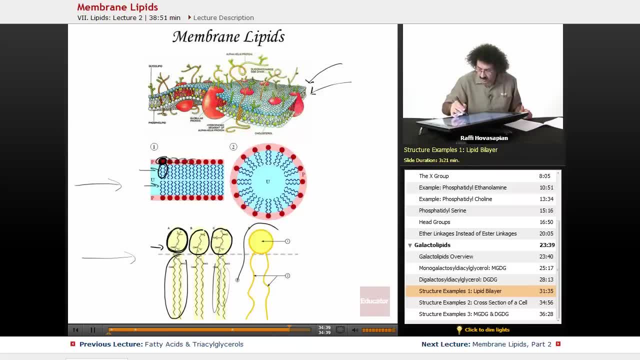 and phosphatidyl ethanol amine and phosphatidyl ethanol amine. phosphatidyl choline. this is the general phosphatidyl choline. this is the general phosphatidyl choline. this is the general structure. this is what you see. this is. 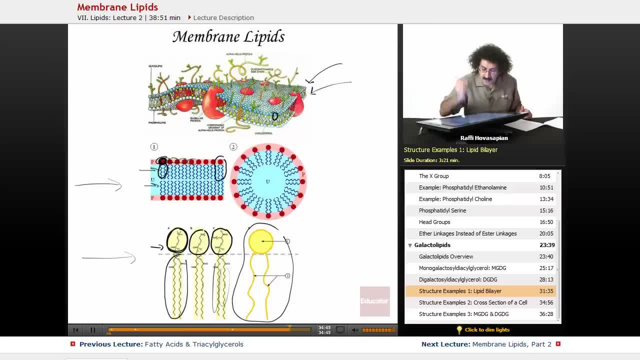 structure. this is what you see. this is structure. this is what you see. this is one of these, is one of these. there you. one of these is one of these. there you. one of these is one of these. there you. now we're just getting into the actual. 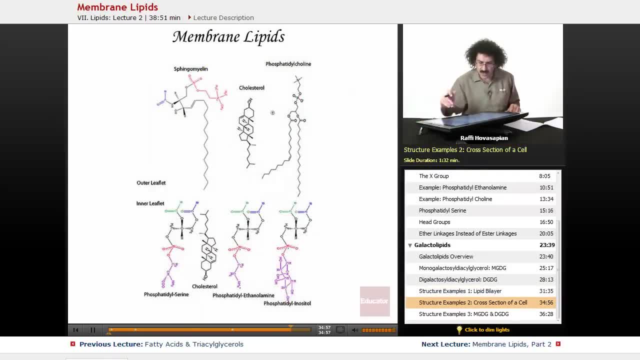 now we're just getting into the actual, now we're just getting into the actual structure of these lipids. okay, so this structure of these lipids, okay, so this structure of these lipids, okay. so this is a nice blown-up view of a cross, is a nice blown-up view of a cross. 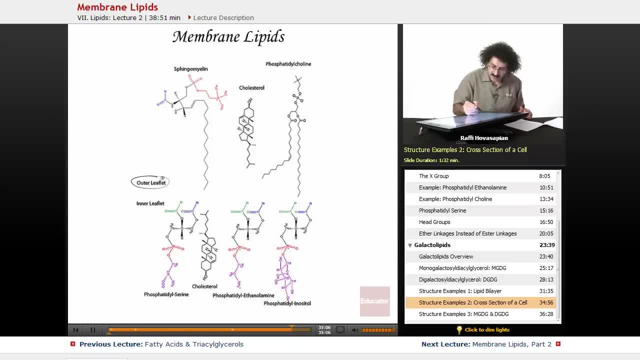 is a nice blown-up view of a cross section of a cell. so in the outer section of a cell. so in the outer section of a cell. so in the outer leaflet, the inner leaflet. so let me go. leaflet the inner leaflet, so let me go. 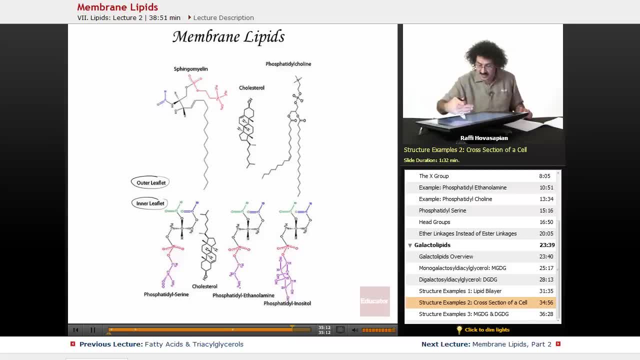 leaflet, the inner leaflet. so let me go ahead and go to blue, so in the outside ahead, and go to blue, so in the outside ahead, and go to blue, so in the outside of the cell, the inside of the cell, so of the cell, the inside of the cell, so 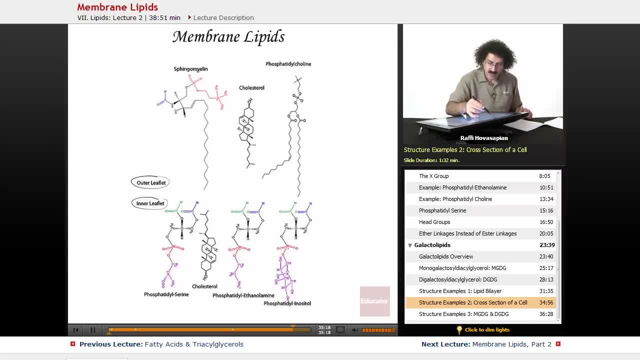 of the cell, the inside of the cell. so this is going to be. let's see sphingo. this is going to be. let's see sphingo. this is going to be. let's see sphingo. myelin cholesterol, so phosphatidyl. myelin cholesterol, so phosphatidyl. 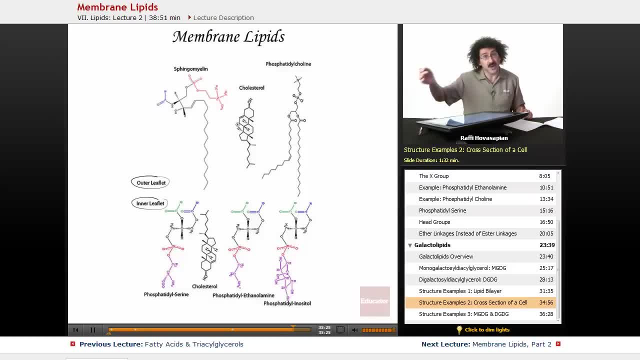 myelin cholesterol. so phosphatidyl choline, a couple of these. we actually choline. a couple of these. we actually choline. a couple of these we actually haven't talked about yet they're going, haven't talked about yet they're going, haven't talked about yet they're going to be the other classes that we're going. 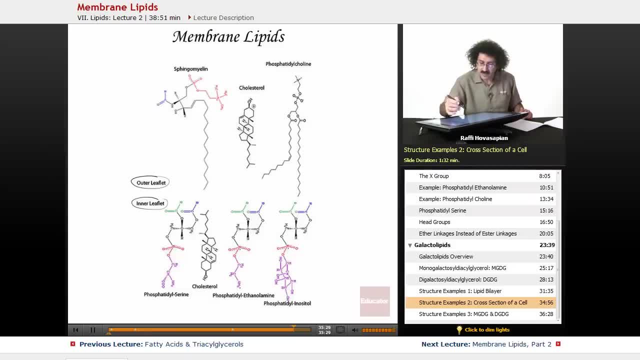 to be the other classes, that we're going to be the other classes that we're going to talk about the sphingo lipids and to talk about the sphingo lipids, and to talk about the sphingo lipids and the sterols, but this one we've talked. 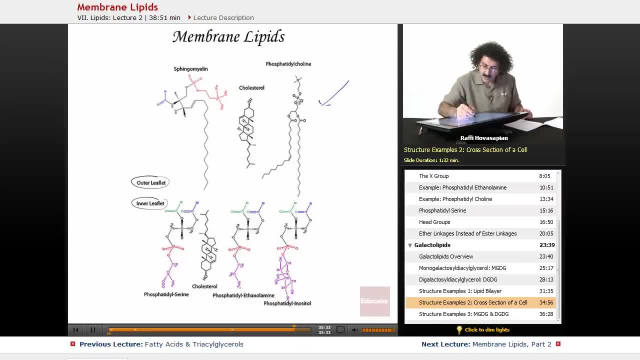 the sterols, but this one we've talked the sterols, but this one we've talked about. so here you have your glycerol, you about. so here you have your glycerol, you about. so here you have your glycerol, you have your phosphate, you have your choline. 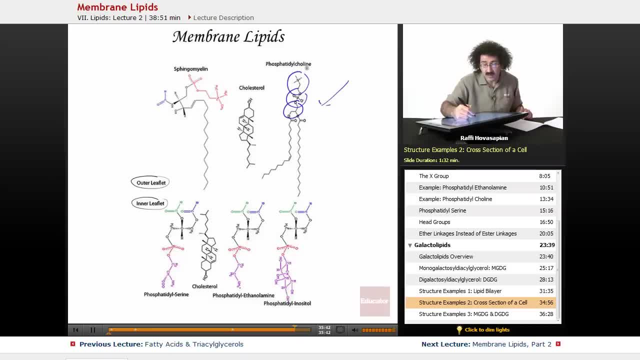 have your phosphate, you have your choline. have your phosphate, you have your choline. okay, so this is the outer leaflet of. okay. so this is the outer leaflet of okay. so this is the outer leaflet of the membrane. inner leaflet of the membrane. 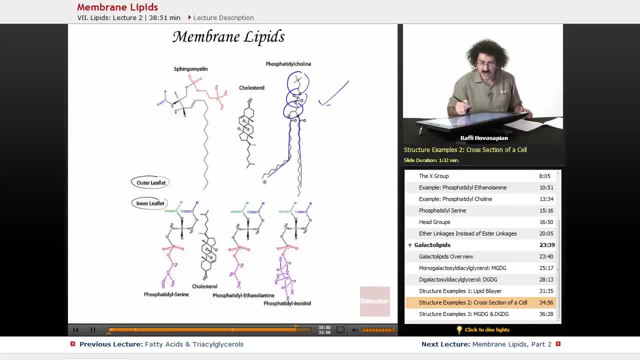 the membrane: inner leaflet of the membrane. the membrane: inner leaflet of the membrane. and then, of course, you have your, and then of course, you have your, and then of course you have your tail group, and of course you have your tail tail group, and of course you have your tail. 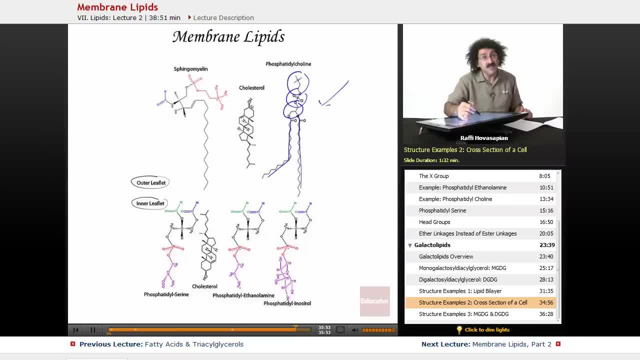 tail group and of course, you have your tail group and these are just some other group, and these are just some other group and these are just some other lipids, some other fats that are actually lipids, some other fats that are actually lipids, some other fats that are actually well, shouldn't call them fat, let's just well, shouldn't call them fat, let's just well shouldn't call them fat, let's just call them lipids. some other lipids that call them lipids. some other lipids that call them lipids. some other lipids that are in the outer leaflet, which we'll 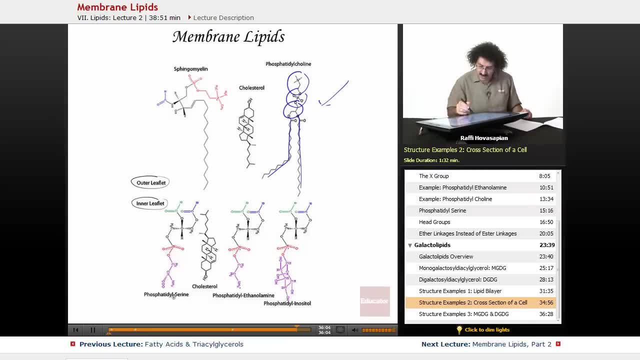 are in the outer leaflet which we'll are in the outer leaflet which we'll talk about in just a little bit. here we talk about in just a little bit. here we talk about in just a little bit. here we have our phosphatidyl serine. here we 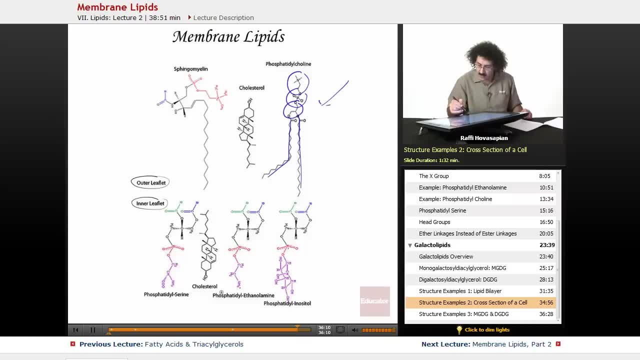 have our phosphatidyl serine here. we have our phosphatidyl serine here. we have another cholesterol. we have have another cholesterol. we have have another cholesterol. we have phosphatidyl ethanolamine and we have phosphatidyl cholesterol, we have. 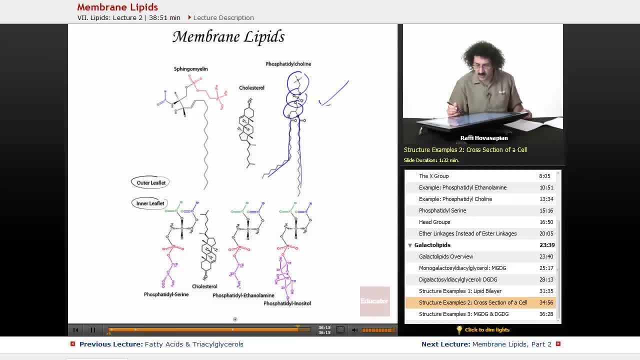 phosphatidyl cholesterol. we have phosphatidyl inositol, which again we'll, phosphatidyl inositol, which again we'll, phosphatidyl inositol, which again we'll talk about in subsequent lessons. so talk about in subsequent lessons. so 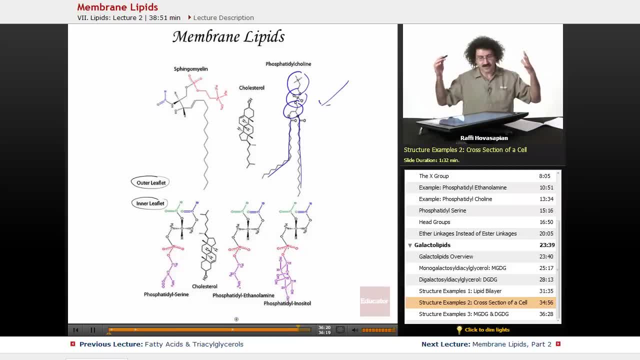 talk about in subsequent lessons. so that's it. it's just an arrangement of that's it. it's just an arrangement of that's it. it's just an arrangement of these lipids, the various lipid classes, these lipids, the various lipid classes, these lipids, the various lipid classes, arranging themselves and making up the 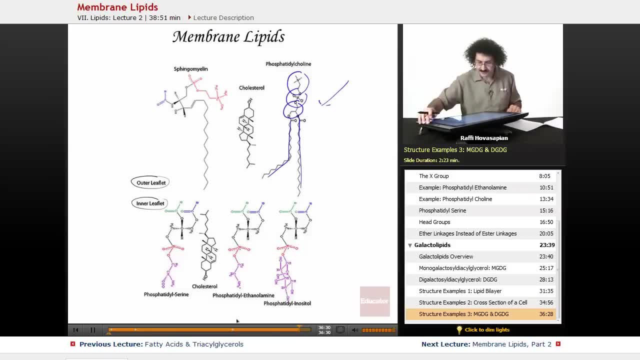 arranging themselves and making up the arranging themselves and making up the cell membrane, that's all okay. a couple cell membrane, that's all okay. a couple cell membrane, that's all okay. a couple of structures here, so that here we have of structures here, so that here we have. 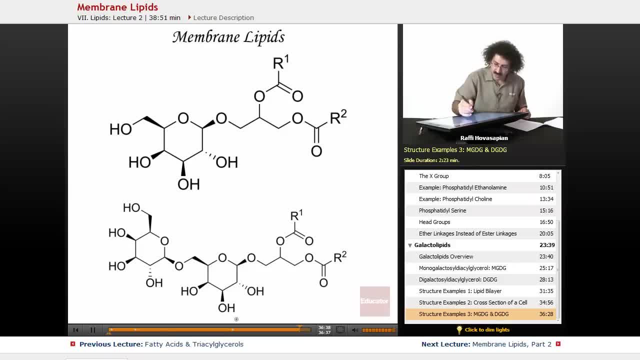 of structures here, so that here we have a mono galactolipid. this one is a mono a mono galactolipid. this one is a mono a mono galactolipid. this one is a mono galactolipid. so this is the MG DG. okay. 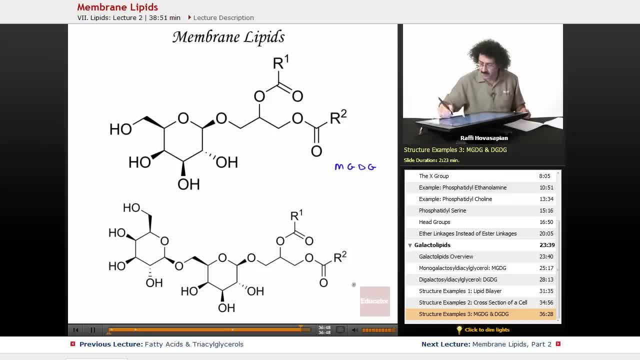 galactolipid, so this is the MG DG, okay. galactolipid, so this is the MG DG, okay. or the mono galacto diacylglycerol- this, or the mono galacto diacylglycerol- this, or the mono galacto diacylglycerol- this is the di galacto diacylglycerol- this is. 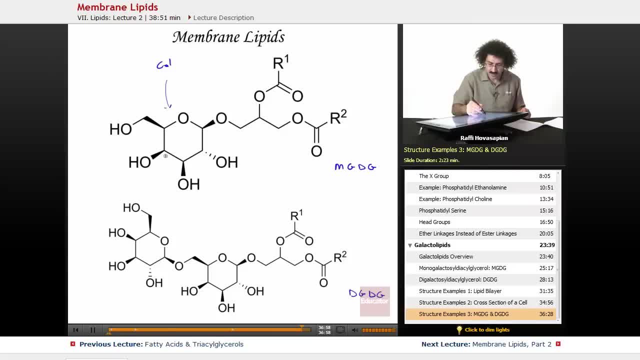 is the di galacto diacylglycerol. this is is the di galacto diacylglycerol. this is our galactose monomer down, up, down, down. our galactose monomer down, up, down, down. our galactose monomer down, up, down, down. now notice, in this particular case, they 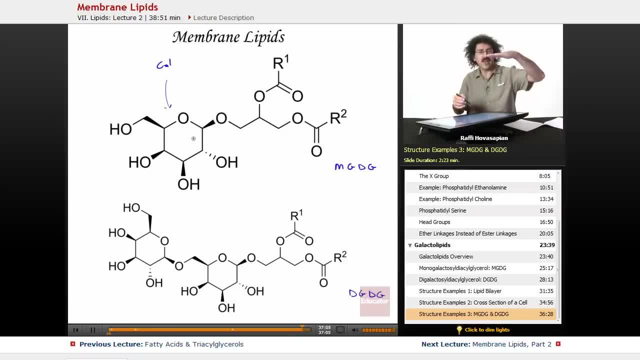 now notice in this particular case. they now notice in this particular case, they actually show you the stereochemistry in. actually show you the stereochemistry in. actually show you the stereochemistry in a different way instead of looking at it, a different way instead of looking at it. 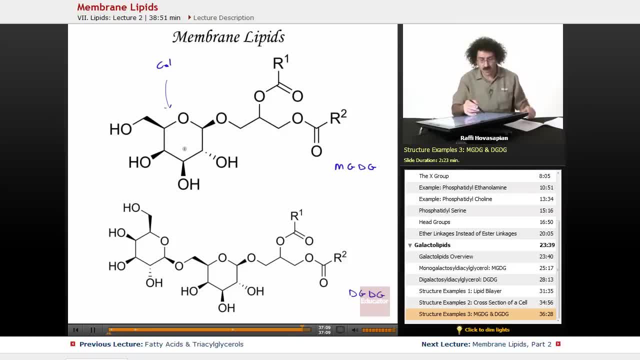 a different way. instead of looking at it in Haworth projection, they're looking at in Haworth projection, they're looking at in Haworth projection. they're looking at it directly like this. so again, just it, directly like this. so again, just it, directly like this. so again, just another way of looking at the molecular. 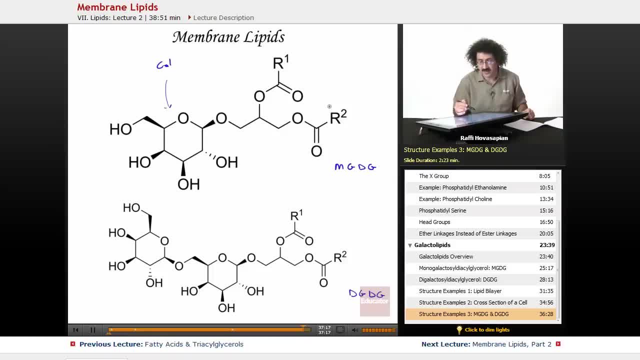 another way of looking at the molecular, another way of looking at the molecular structure of something. you're gonna structure of something. you're gonna structure of something. you're gonna often see structures like this. that's often see structures like this. that's often see structures like this. that's the thing with biochemistry- different. 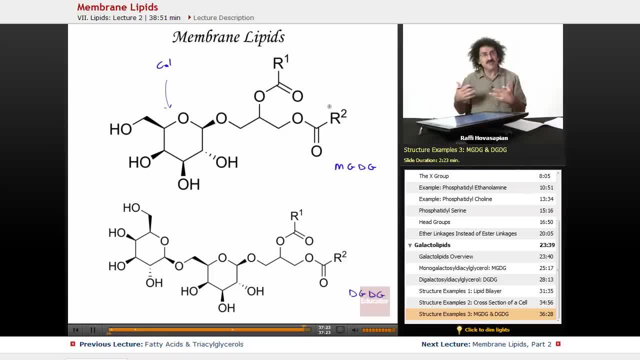 the thing with biochemistry: different the thing with biochemistry: different projections, different views. give us projections. different views give us projections. different views give us different bits of information. so just different bits of information. so just different bits of information. so just wanted you to see something a little bit. 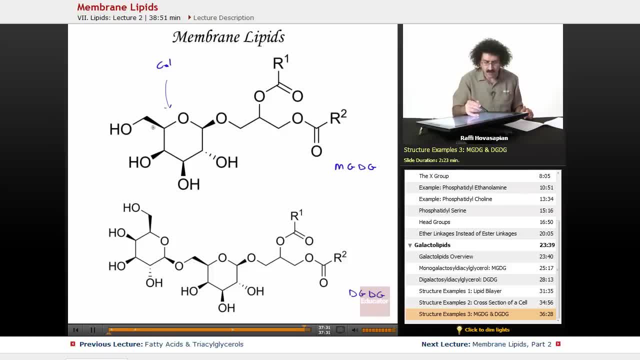 wanted you to see something a little bit. wanted you to see something a little bit different than a Haworth projection back, different than a Haworth projection back, different than a Haworth projection back. forward, forward, forward. here we have our, forward, forward forward. here we have our. 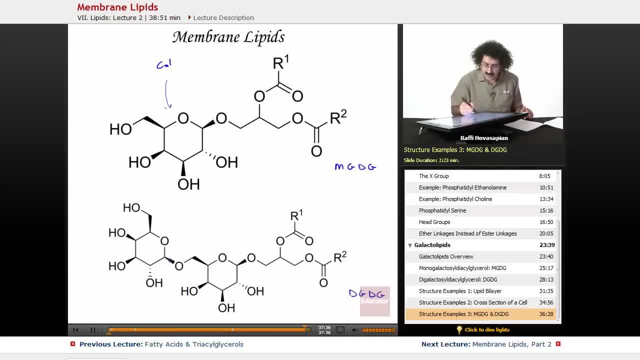 forward, forward forward. here we have our two galactose monomers. they are connected, two galactose monomers. they are connected, two galactose monomers. they are connected in what we said was alpha 1- 6, because in what we said was alpha 1- 6, because 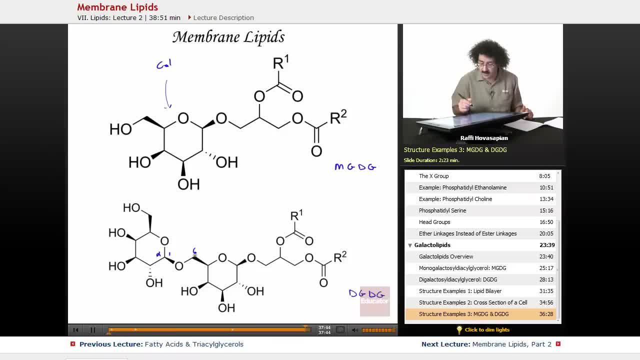 in what we said was alpha 1, 6, because this is the 1, 2, 3, 4, 5, 6 carbon right. this is the 1- 2, 3, 4, 5, 6 carbon right. this is the 1- 2, 3, 4, 5, 6 carbon right. there, this is going to be a beta 1. 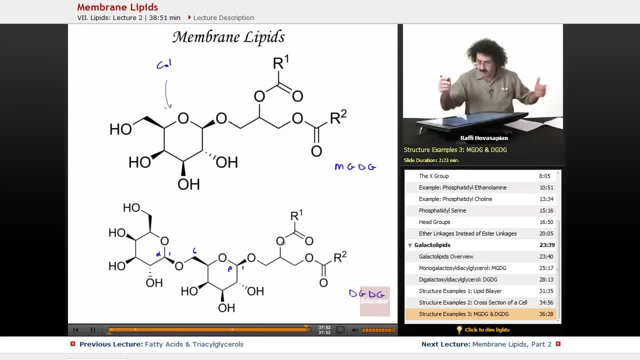 there this is going to be a beta 1. there this is going to be a beta 1 connection to glycerol. so that's it just connection to glycerol. so that's it just connection to glycerol. so that's it. just wanted you to see. you know what it is. 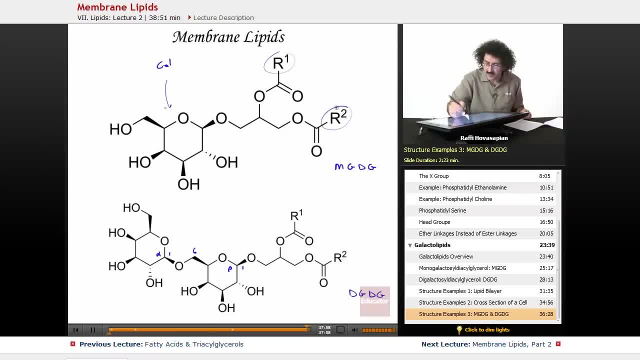 wanted you to see you know what it is, wanted you to see you know what it is that they actually looked like. these, are that they actually looked like? these are that they actually looked like? these are our acyl groups. again, r1 and r2 tend to 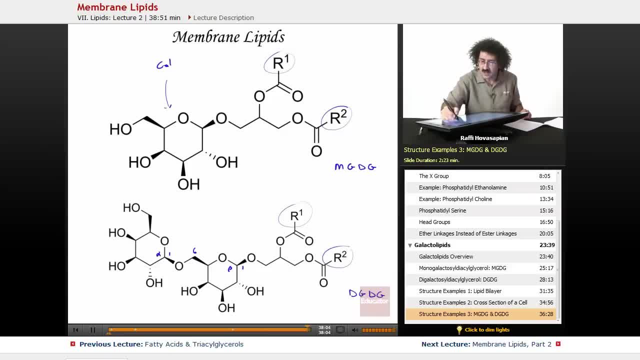 our acyl groups again. r1 and r2 tend to our acyl groups again. r1 and r2 tend to be the same. but they don't have to be be the same. but they don't have to be be the same, but they don't have to be the same. so we left it that way we have. 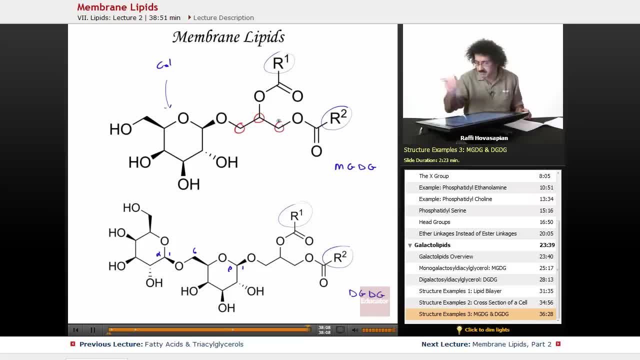 the same, so we left it that way. we have the same, so we left it that way. we have our glycerol, which was carbon 1, carbon 2. our glycerol which was carbon 1, carbon 2. our glycerol which was carbon 1, carbon 2, carbon 3, or 1, 2, 3, however you want to. 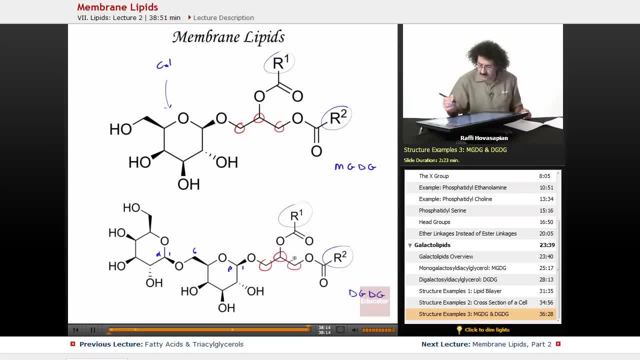 carbon 3 or 1 2, 3, however you want to. carbon 3 or 1 2, 3, however you want to arrange it: 1 2, 3. ester linkage ester. arrange it: 1, 2, 3. ester linkage ester.